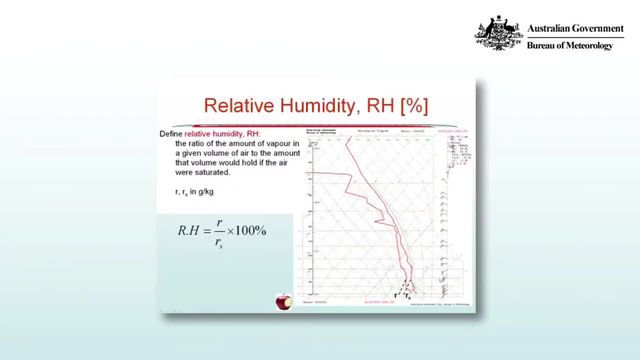 Relative humidity. Relative humidity is a fairly familiar concept to most people and it's a common parameter to work out, to calculate in meteorology, as a measure of the degree of saturation of an air mass. So let's define relative humidity in percentage as the ratio of the amount of vapour in a given volume of air to the amount that volume would hold if the air were saturated. 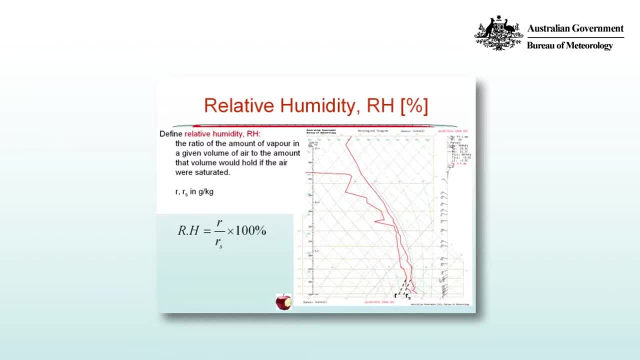 So we may write: relative humidity is R, the mixing ratio in grams per kilogram divided by RS, the saturation mixing ratio in grams per kilogram multiplied by 100.. And the convenience of using the mixing ratio is that the mixing ratio can be obtained from the dew point profile, the saturation mixing ratio from the temperature profile, and that's very easy to do on a skew. T log P aerological diagram. 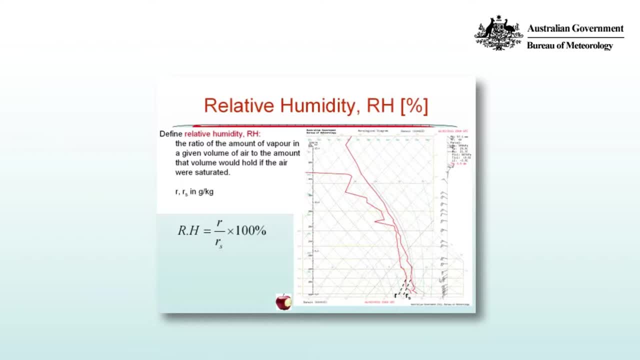 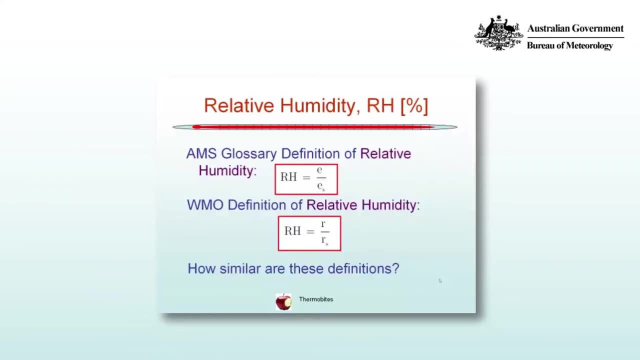 And even just visually, you can see, By the degree of closeness between the temperature and the dew point temperature profile, whether or not the air is close to saturation. However, there are two ways of defining relative humidity. The American Met Society glossary defines relative humidity as the ratio of the vapour pressures, whereas the World Meteorological Organization defines, as we've just done, the relative humidity as the ratio of the mixing ratios. 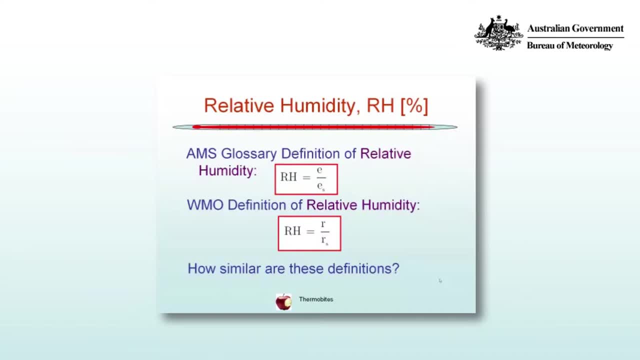 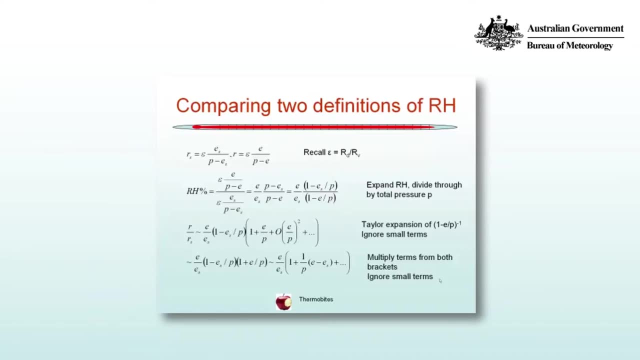 So how similar are these definitions? Does it really matter which one we use? Well, again a little bit of math. So if you need to, I'm going to stop the video and work this out. fine, As we've seen earlier, the mixing ratios may be expressed in terms of this ratio of the specific gas constants or the molecular weights between dry air and water vapour, and in terms of the relevant vapour pressure and the total pressure P. in those two expressions there 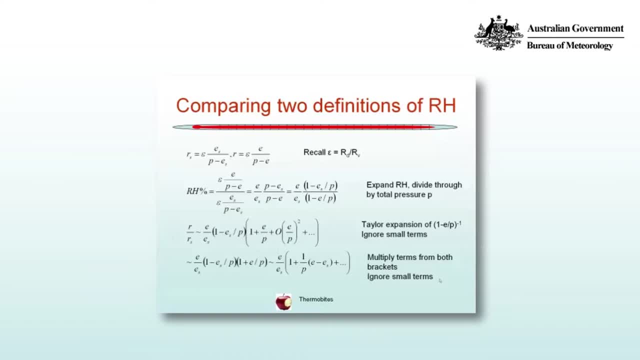